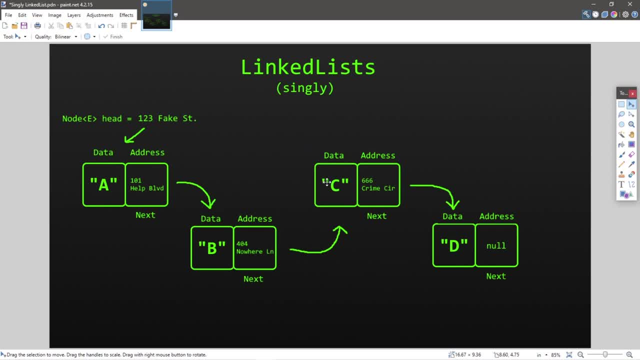 chain of nodes. Each node contains two parts: some data that we need to store and an address to the next node in line, also referred to as a pointer. Linked lists do not have an index the same way that arrays do, but each node contains an address to where the next node is located. So these nodes- 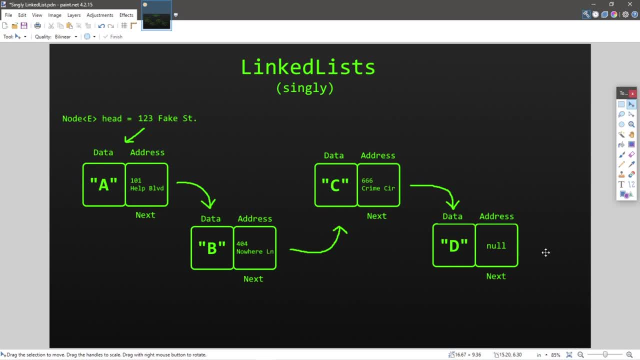 are non-contiguous. They can really be anywhere within your computer's memory. If our initial node has a memory address of 123 Fake Street, like our array example, then the next node in our linked list could have a memory address of maybe 101 Help Boulevard and another could be 404, Nowhere Lane. 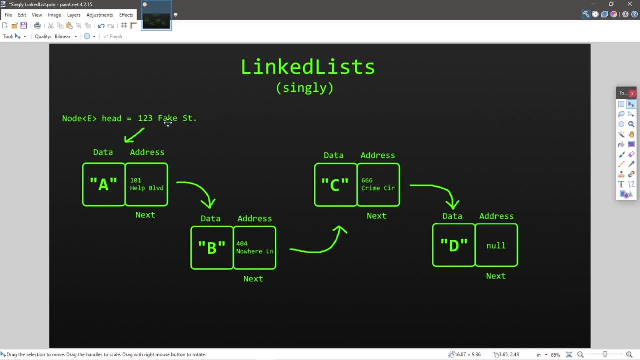 and another could be 406 Crime Circle. Each node knows where the next node resides. I imagine this as if we're following a scavenger hunt or a series of clues to find the end of the linked list, the tail. Each node has an address, a clue as to where the next node is. We begin at the head. 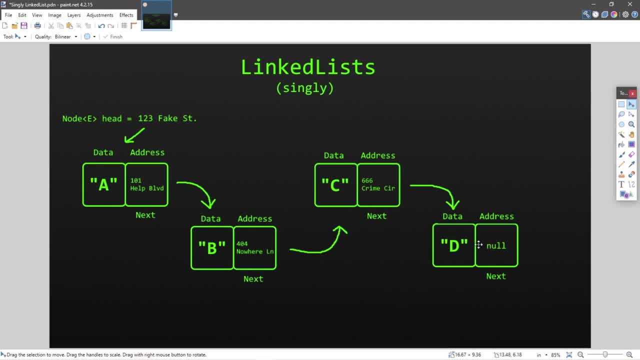 and work our way towards the tail, following each clue, each memory address found in each node. Then we know when we reach the end of our linked list. when we check that address, our pointer, and it has a value of null, That means we're at the tail, we're at the end of our linked. 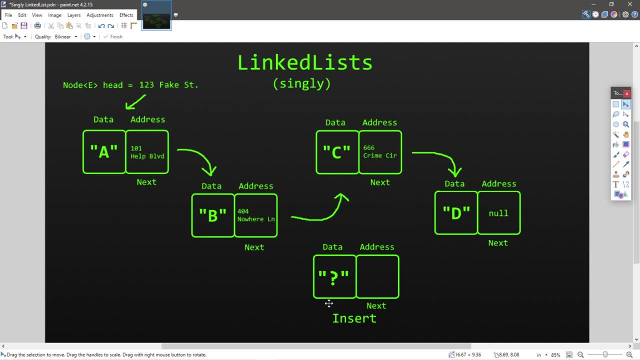 list. Now. inserting a node is easy in a linked list. There's no shifting of elements involved. Wherever we need to place a new node, we take the address stored in the previous node and assign the address of our new node with the address from the previous node, so that our new 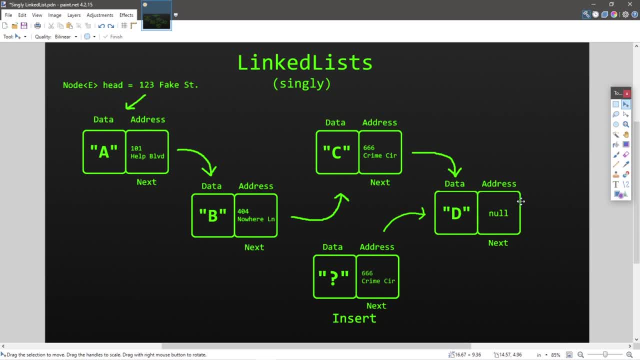 node is pointing to the next node in line, Then we can take and replace the address in the previous node with an address that points to our new node. It's as simple as that and we're completing our chain simply by inserting a node at a given location. There's only a few steps involved. 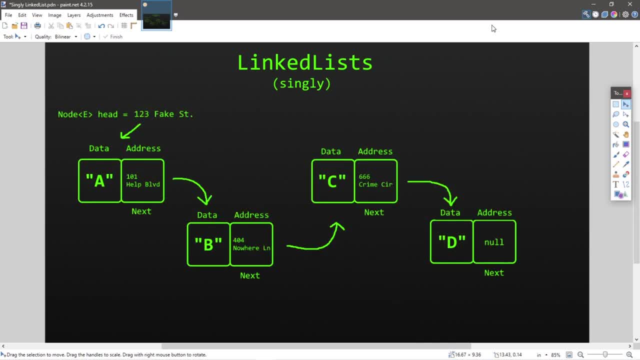 no shifting of elements. So let's go ahead and start the node. We'll start our new node by deleting a node. Deleting nodes are easy too. Wherever we need to delete a node, we have the previous node point instead to the next node in line. Again, no shifting of elements is necessary. 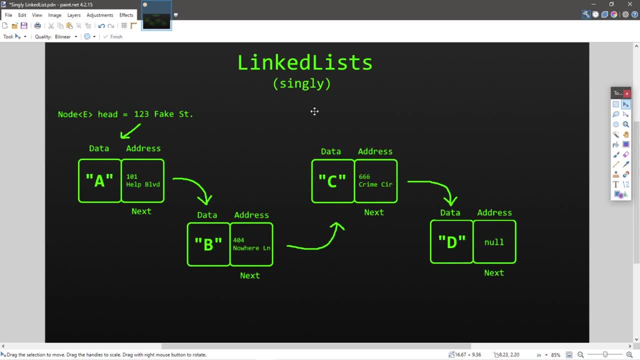 Now this is where linked lists tend to be inferior to arrays. They are bad at searching. We can randomly access an element of an array because we have an index With a linked list. that is not the case. To locate an element, we need to begin at the head and work our way towards the tail. 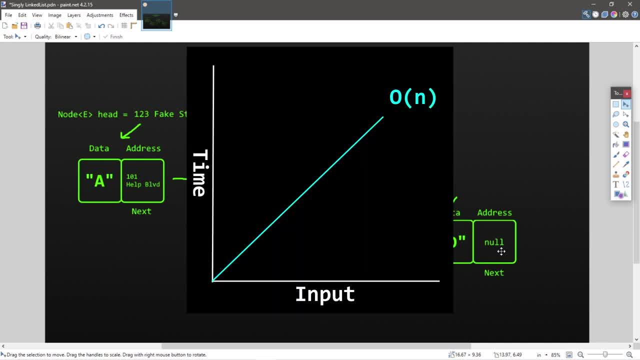 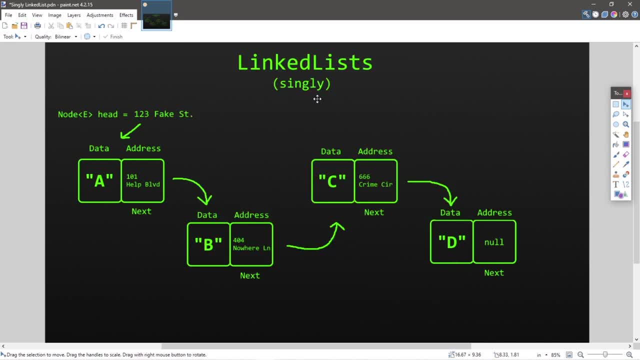 until we find the element that we are looking for. This itself takes time. In fact, it would take linear time, but making the insertion or deletion of a node is constant. This variation of a linked list is a singly linked list. There are single links to each node. However, there's another. 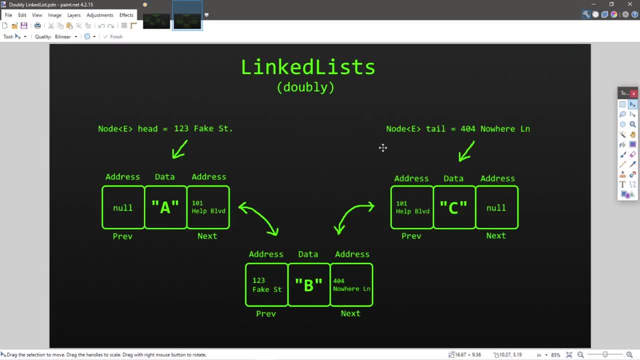 variation called a doubly linked list. A doubly linked list requires even more memory to store two addresses in each node, not just one, which is the case with a singly linked list. One address for the next node and another for the previous node in our chain. 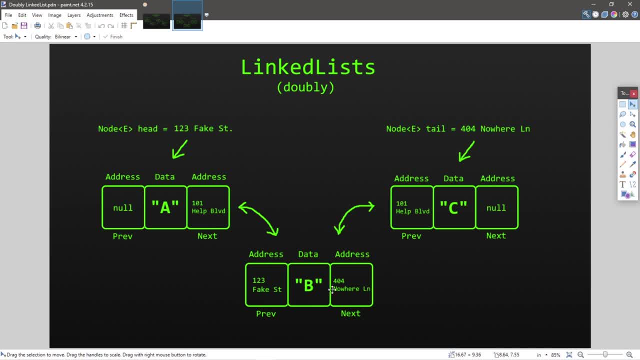 The benefit of a doubly linked list is that we can traverse our doubly linked list from head to tail or from tail to head in reverse. Each node knows where the next and previous node is. but the downside is that a doubly linked list uses even more memory than 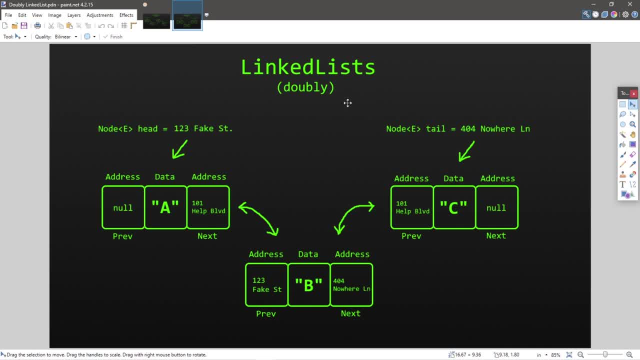 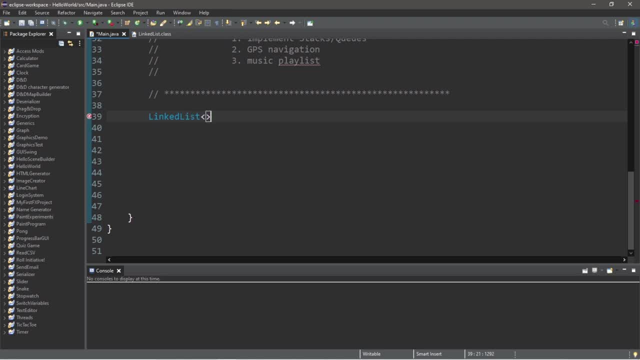 a singly linked list. So how about we create a linked list in real life? now? Let's do it. All right, ladies and gentlemen. with all that out of the way, let's create a linked list. Linked list lists the data type of the objects we'll be storing within this linked list. 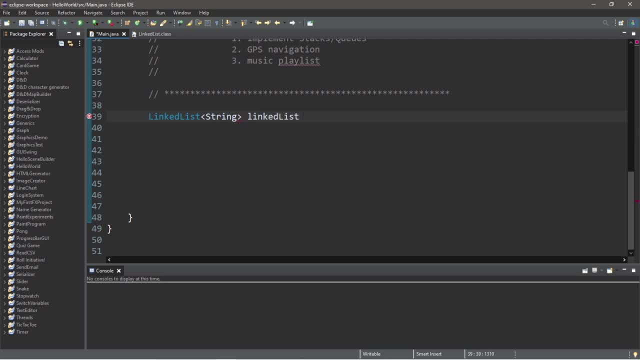 just strings because they're easy, and I will name this linked list linked list. Linked list equals new linked list and list the data type. Again, we are storing strings at a constructor. Boom, you got yourself a linked list. Now if I was to take my cursor and hover over my linked list? 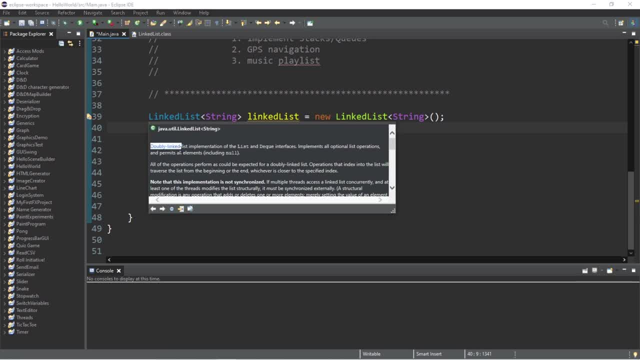 declaration. there's a note here that says this is a doubly linked list. Each node knows where the previous and next nodes are. Now, if we head to the linked list class itself, there's a few things I need to mention here. Our linked list stores the memory location of 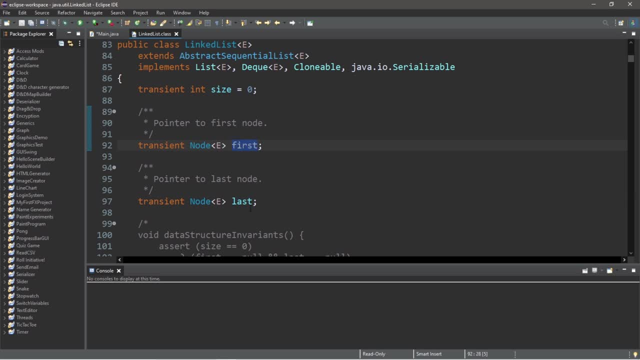 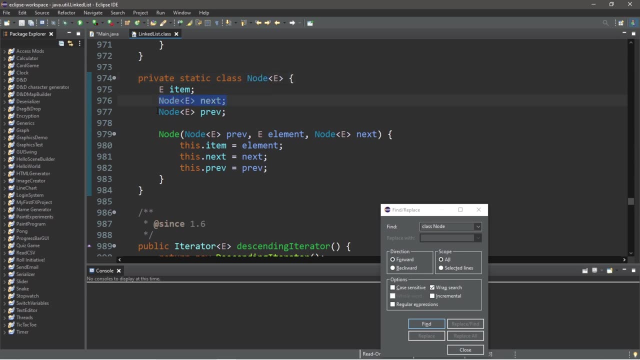 our first and last nodes. These are effectively the head and the tail of our linked list And there's also an inner class named node. Each node knows the memory address of the next and previous nodes within this linked list. Now taking a look at our linked list, class. 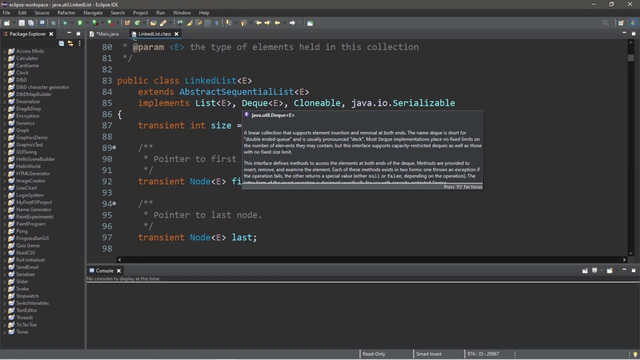 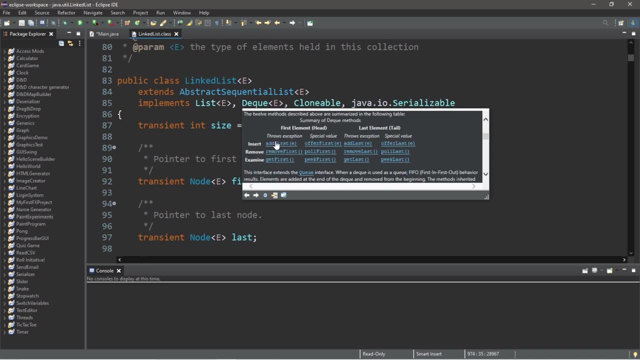 definition. our linked list class implements the deck interface and a deck is more or less a double-ended queue. So with the deck interface we implement 12 additional methods. So here's just a few of them So we can add to the head, add to the tail. remove the head, remove the tail. 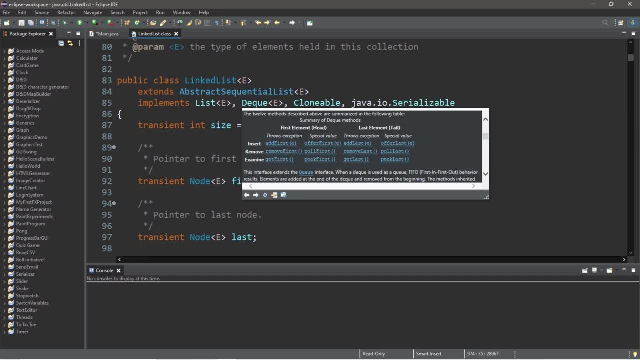 peek at the head, peek at the tail. remove the tail. peek at the head, peek at the tail, peek at the tail. Some will throw exceptions, some will return a special value. So you can use any combination of these, really, And not only do we have these 12 methods, but we can treat our 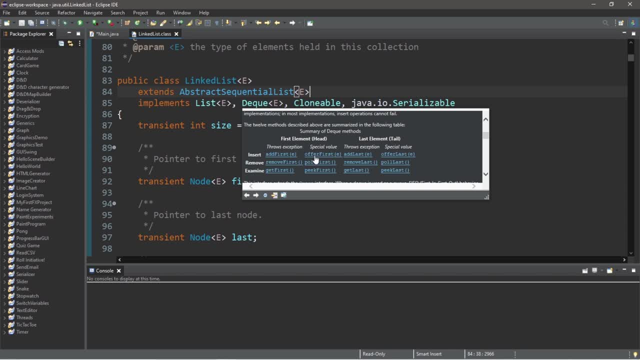 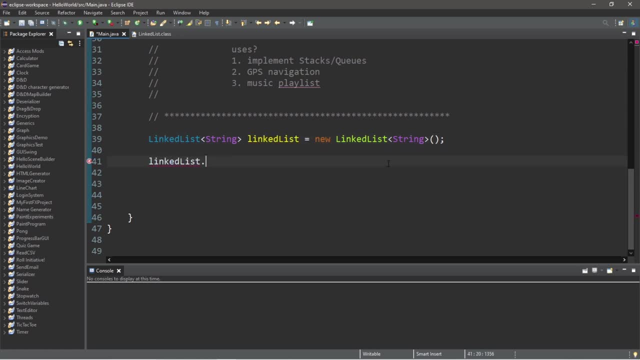 linked list as either a stack or a queue. We can push, we can pop, we can pull and we can offer. So just to demonstrate, let's first treat our linked list as a stack, So linked lists do have a push method as well. if we need to push an element onto our linked list as if it were a 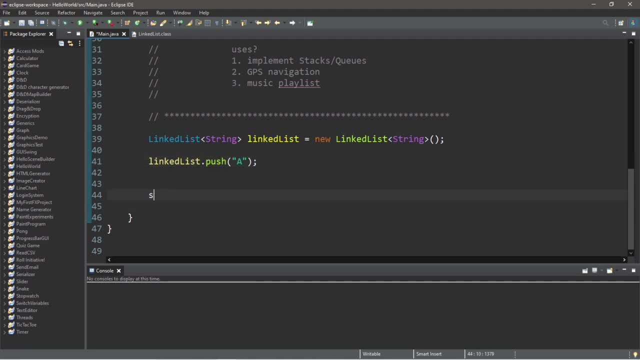 stack. So let's push the letter A and then I will display my linked list with a print line statement: Systemoutprintln linked list. and of course we have the letter A. So let's push another letter onto our stack. What about B? So at the bottom of our linked list we have A. 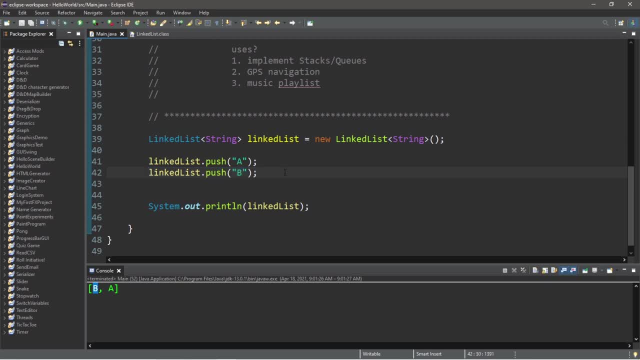 and then on top we have B. Let's add a couple more letters. Let's represent a typical grading scale. We have C, D and F. A, B, C, D, F- Notice that I'm intentionally leaving out E. We're going. 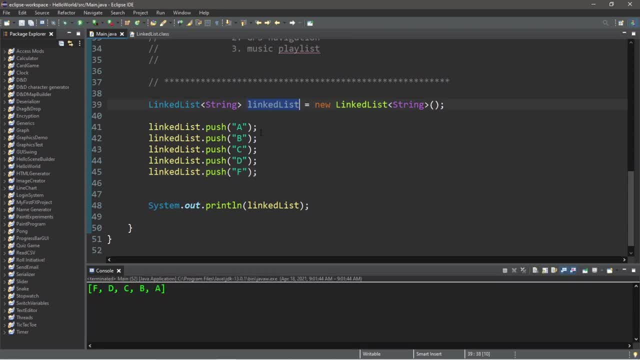 to insert that later. So within our linked list that's behaving as a stack. we have F on top, then D, C, B and A. So we also have access to a pop method as well. Linked list, dot pop and this will pop the top of my linked list. So F should no longer be here, It's D, C, B and A. 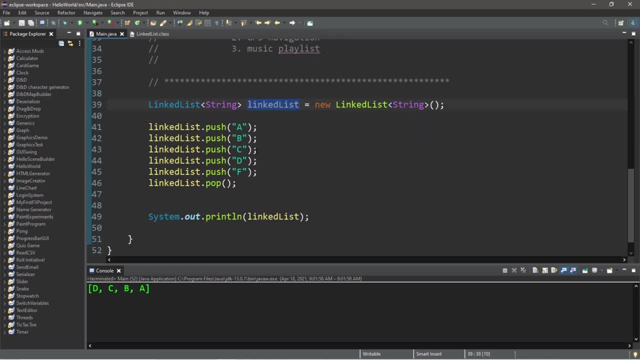 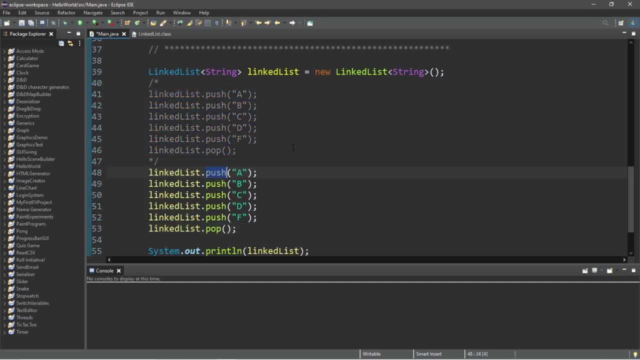 So we can treat a linked list as a stack, We can also treat it as a queue as well, And just to save some time, I'm going to copy these lines of code to add an element to a queue. We do not use push, we use offer. So linked list, dot offer. 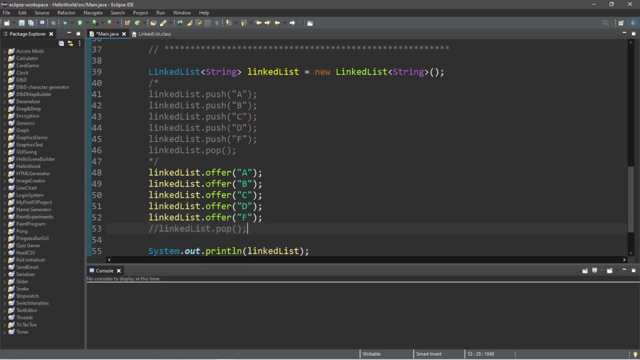 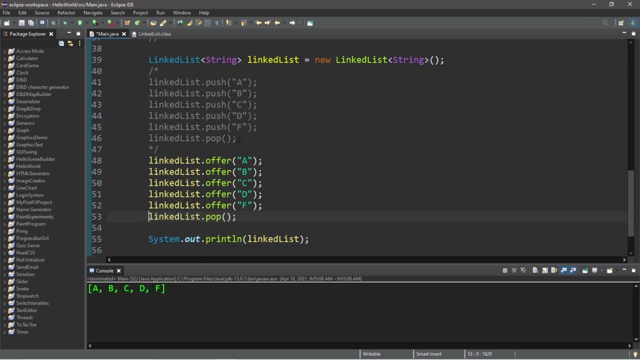 And we will keep the order, So I'm not going to pop it quite yet. So we have A, B, C, D, F. A is at the head, F is at the tail, And to remove the head of our queue: 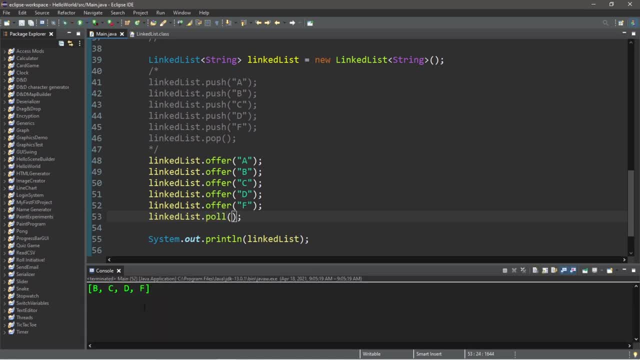 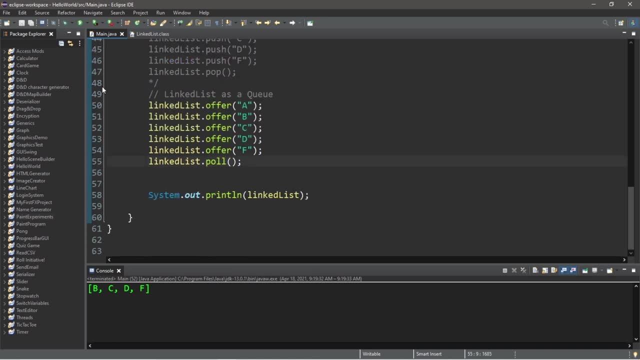 we do not use pop, we use pull, And A is no longer in here. We have B, C, D, F, So you can use a linked list to mimic a stack or a queue. Before we move on to the next section, I'm going. 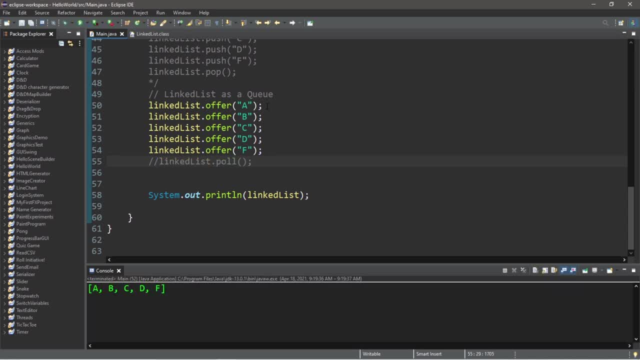 to get rid of this pull method. So we have a typical grading scale: A, B, C, D, F. Where linked lists are really good is the insertion and deletion of nodes. Let's say, for this example, I need to add a node. 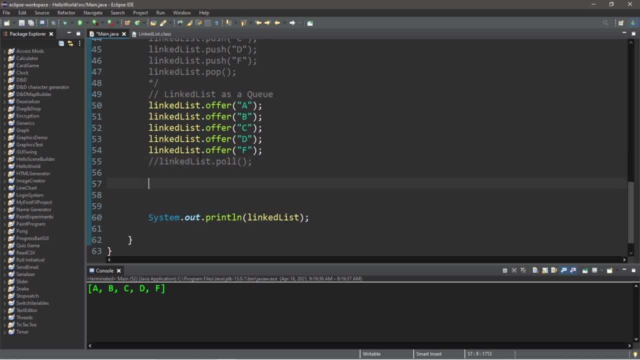 between D and F that contains the letter e. So that's really easy to do. with the linked list, We would type the name of our linked list, dot add, list an index like 4, and our object e. And then to remove a node we would type the name of our linked list, dot remove, then list the. 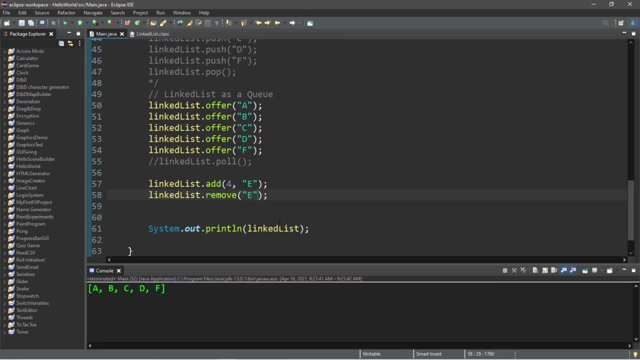 object e. So e should no longer be within my linked list, So where linked lists tend to have an advantage over Christian meinen, united with linked list. e should no longer be at the center of my linked list, So where linked lists tend to have an advantage over other linked lists. 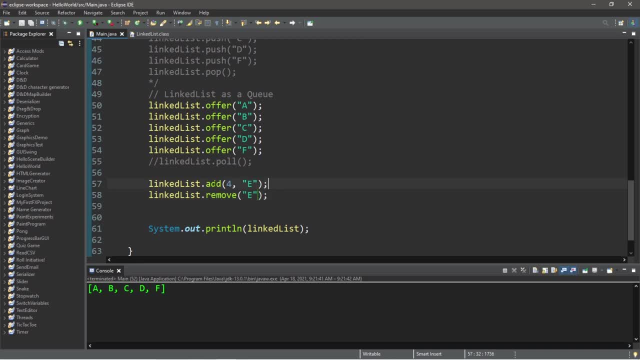 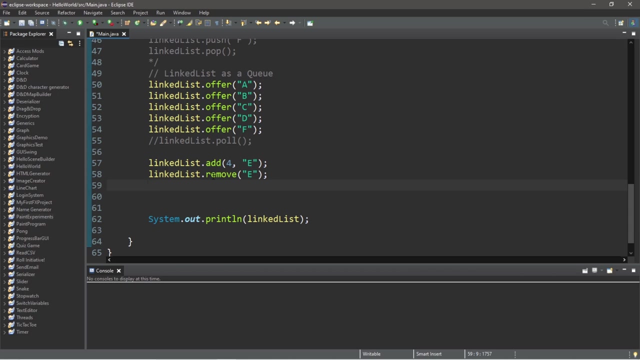 advantage over arrays and array lists is the insertion and deletion of nodes. However, there's one catch to this. With a linked list, we still need to traverse the entire linked list to find where we need to go. Unlike with arrays and array lists, there's no random access to a linked list. Searching for an element is 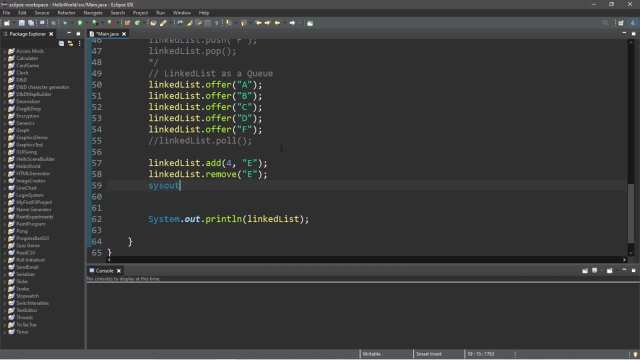 fairly straightforward too. So within a println statement I'm going to use the indexOf method of a linked list: linkedListindex of. let's look for f, So that would be at index 4.. And before we wrap things up here, here's a few methods. 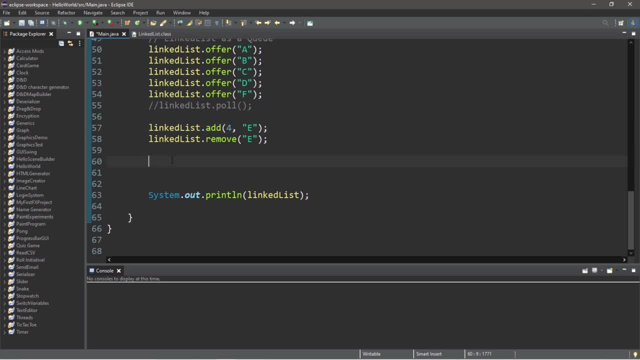 related to linked lists that you might be interested in. We can peek at the head or the tail node of our linked list. So within a println statement I'm going to print linkedList and then use the peekFirst method. So the first. 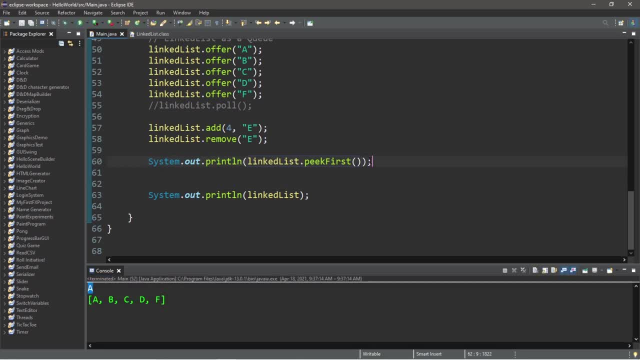 node within my linked list contains the letter a, So we can peek last as well, linkedListpeek Last and the last node of my linked list contains the letter f. we can add new nodes at the head or the tail of our linked list by using the add first method for the head. so maybe i need to add, maybe zero, because i don't. 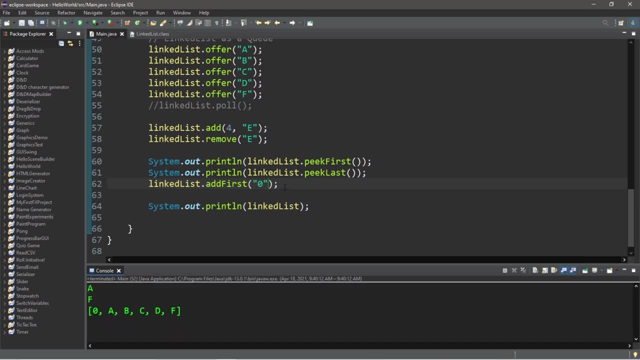 really know what comes before a in the alphabet. so zero would be a good bet, i guess, or we could add to the tail by using add last, and after f comes g, and we now have g at the tail of our linked list. we can remove first and remove last. you can also store them within a variable too. 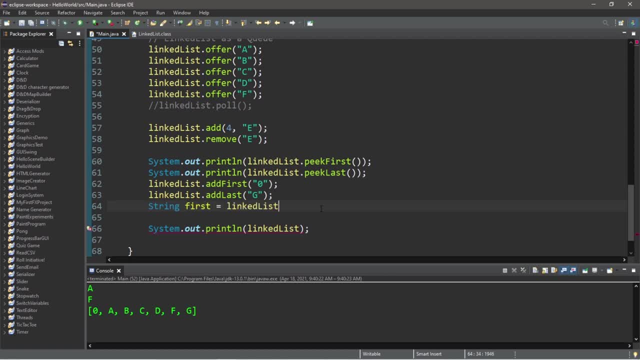 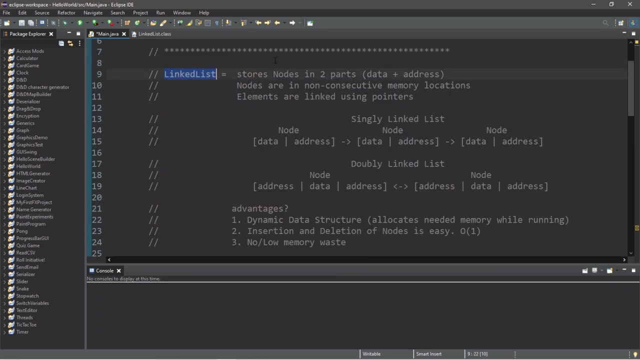 let's say: string first equals linked list dot remove first. then to remove the last node, we could just use remove last. then and let's store this within a different variable: remove last. so yeah, those are a few useful methods related to linked lists. in conclusion, everybody, a linked list is a data. 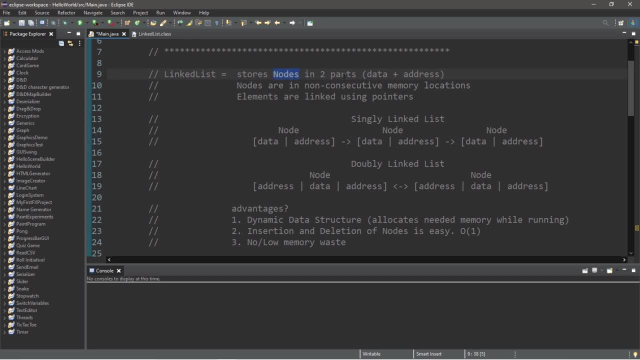 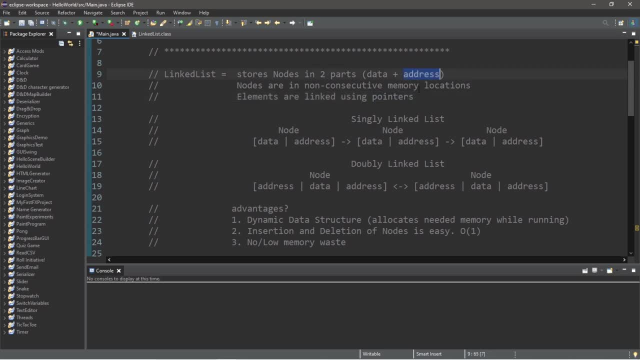 and elements are linked via these pointers. they contain an address for where the next node is. we've discussed two varieties of linked lists: a singly linked list as well as a doubly linked list. with a singly linked list, each node is made up of two parts: some data and an address. two 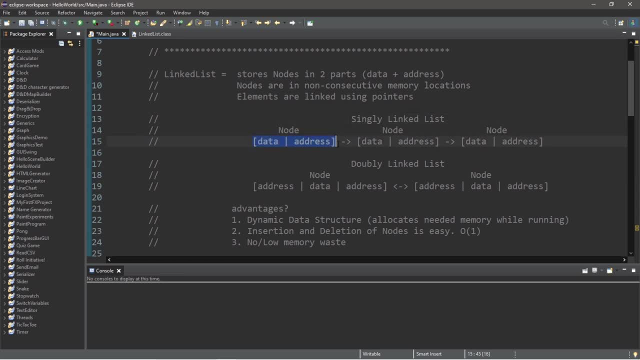 to traverse a singly linked list. we would begin at the head node and use the address as a sort of clue to find where the next node is located within our computer's memory. with a doubly linked list, each node is made up of three parts: some data and two addresses. one address for the next node. 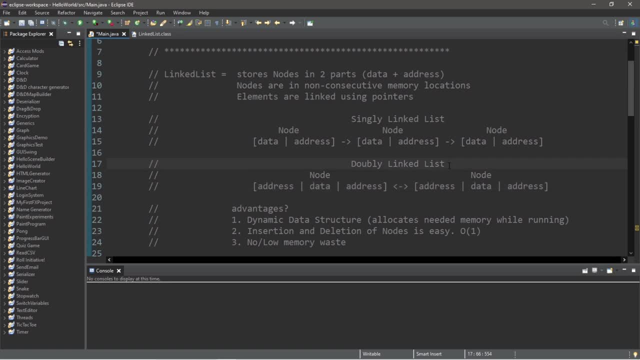 and another address for the previous node and it behaves the same way. and to traverse a doubly linked list, we could begin at the head and work our way towards the tail, or we could begin at the tail and work our way towards the head, depending on which way is closer to where the next node is. 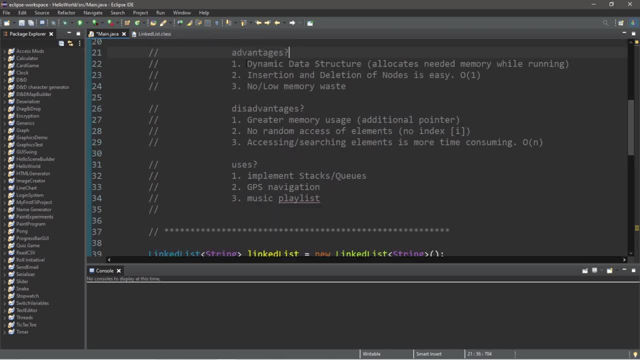 we need to be within our linked list. what are some of the advantages of a linked list? one: they're a dynamic data structure. they can allocate needed memory while their program is currently running. two: insertion and deletion of nodes is really easy if you're familiar with big o notation. this 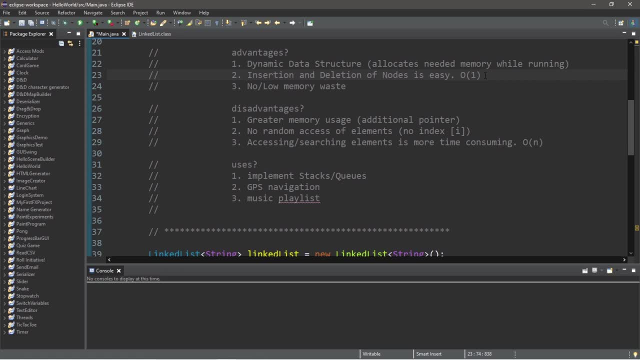 would be in constant time. there's only a few steps, regardless of the size of our data set. and three, there is no to low memory waste. what are some disadvantages? one: there is greater memory usage because we have to store an additional pointer. each node also has a different memory. 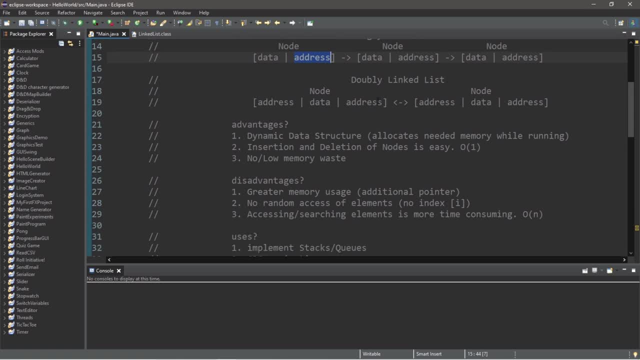 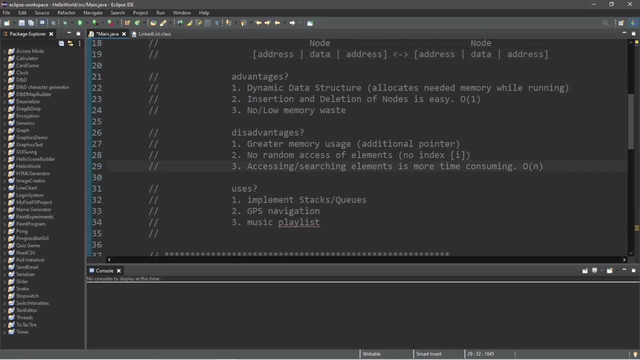 usage because we have to store an additional pointer. each node also has a different memory- also stores the address for where the next node is located and even more so with a doubly linked list, this will use a lot more memory because we need two addresses for each node. now two there's.